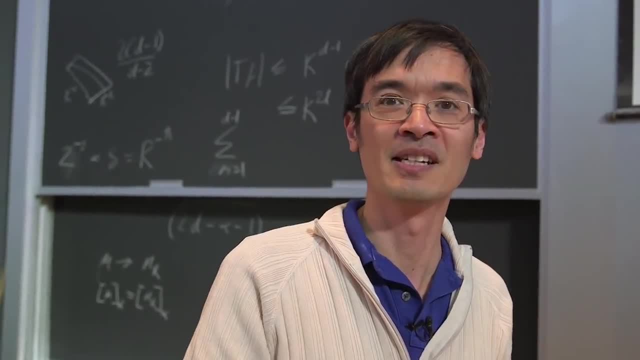 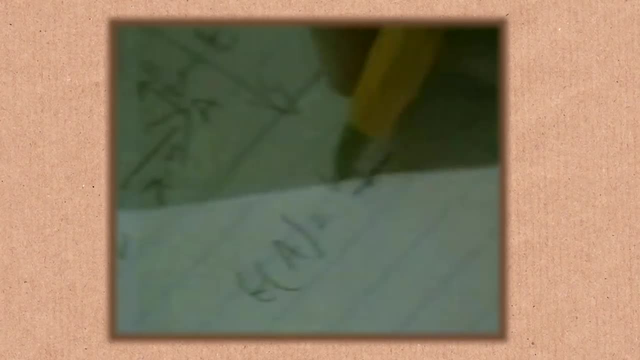 numbers on the. she put the detergent on the windows in the form of numbers. So I always liked numbers and patterns and logic, And so things are very black and white where there's one right answer and everything else is wrong. I didn't like sort of subjective shades of gray type. 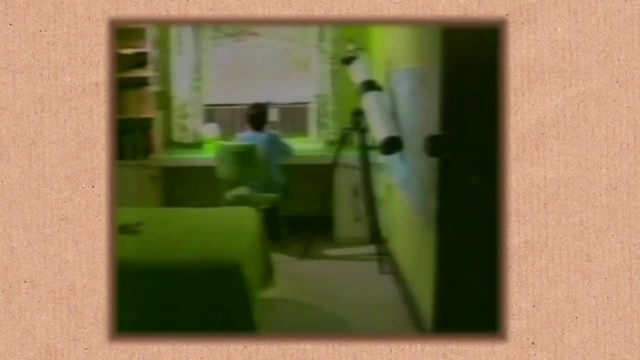 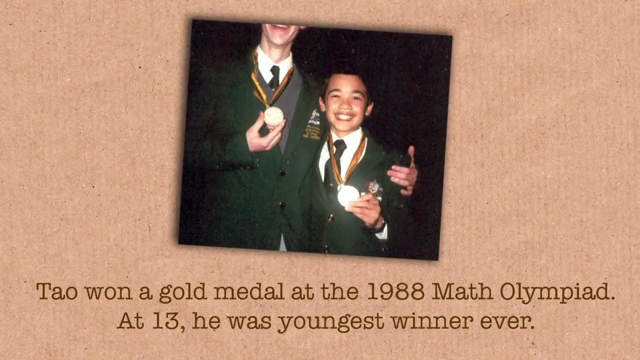 questions. I would work on math workbooks for fun. You know, if my parents wanted to shut me up, just give me a workbook and I would just, you know, do sums and so forth. So I always liked mathematics and math competitions. Doing that was very different. 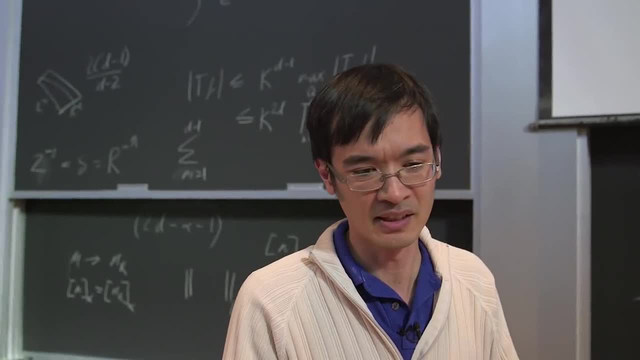 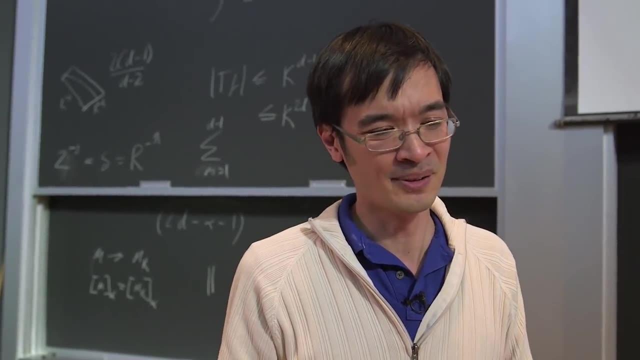 from doing research, mathematics, The type of problems that you're given in a problem book and so forth. these are so very canned problems, things that you can do in five minutes or 10 minutes, And they don't prepare you completely for a research problem where you know you have. 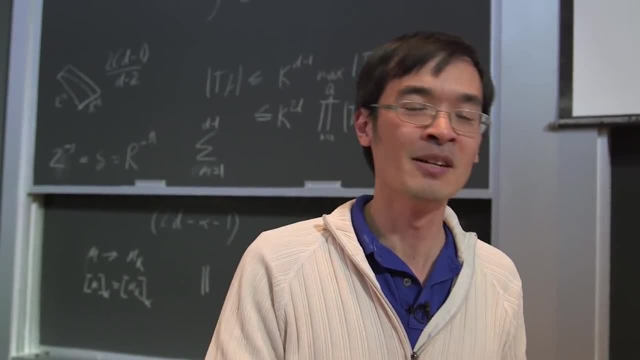 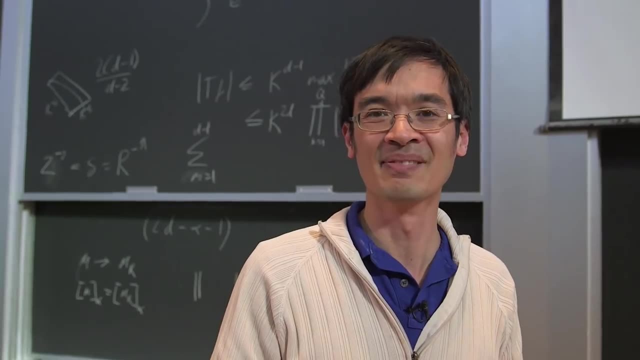 to spend six months. you have to read the literature, talk to people, try something that doesn't work, modify it, try it again, And it's a very different experience doing research, But I like it a lot better actually than all the puzzles I used to do as a kid. I don't 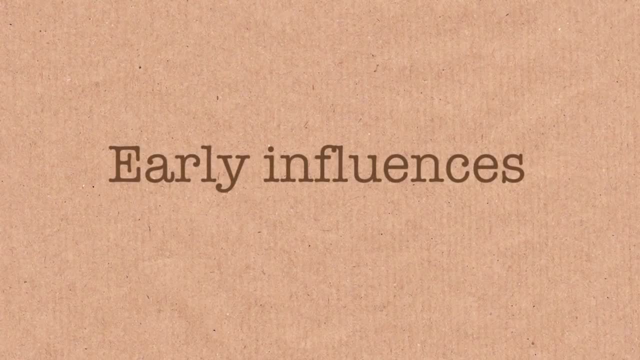 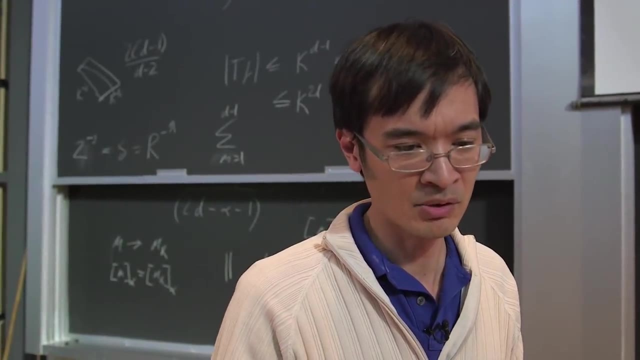 like to do these things very much anymore. My mother was a high school math teacher when she was younger, So she did help me a little bit. you know, when I was a kid, you know just talking numbers with me, And then I had 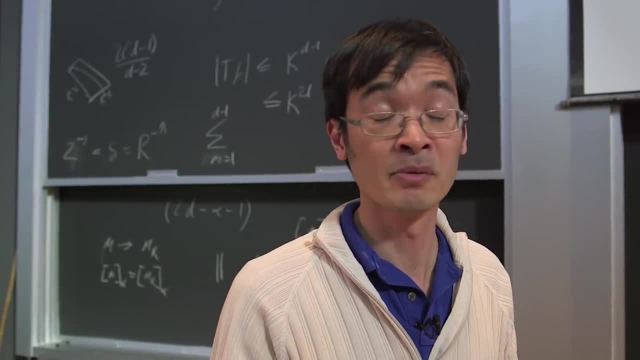 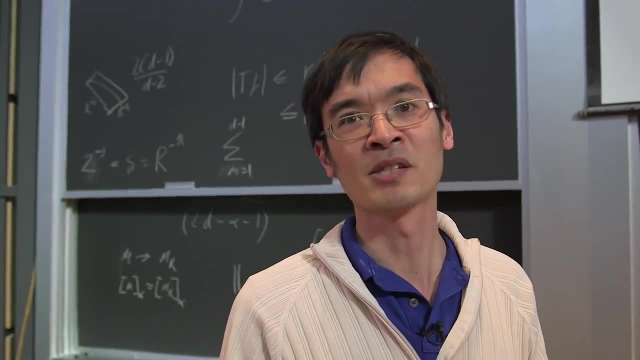 a lot of very good mentors. When I was like 10 or 11, there was a retired math professor in Adelaide which I would go visit on the weekends. We'd have tea and cookies and you know, he would just discuss some recreational math problem and so forth And it was just. 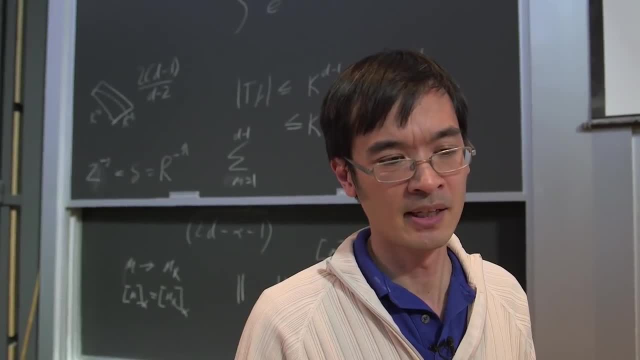 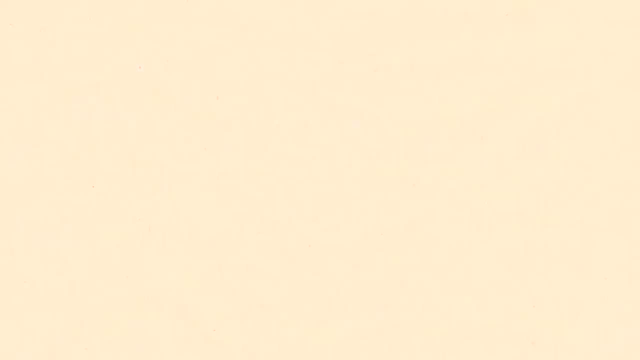 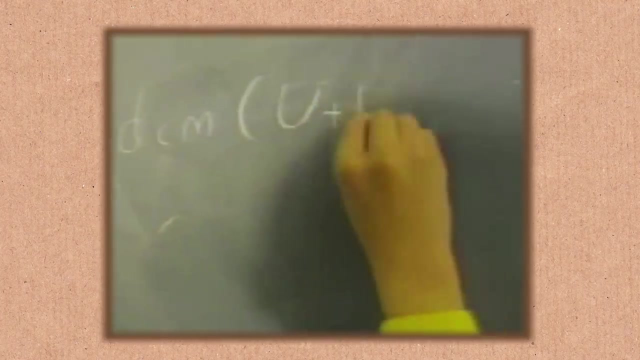 a lot of fun. He would tell me stories about how he used math during World War II, You know, to do ballistics and so forth. It was kind of fun to actually see math actually being used for something. He had a PhD in maths from Princeton at 20 and was appointed Professor of Mathematics. 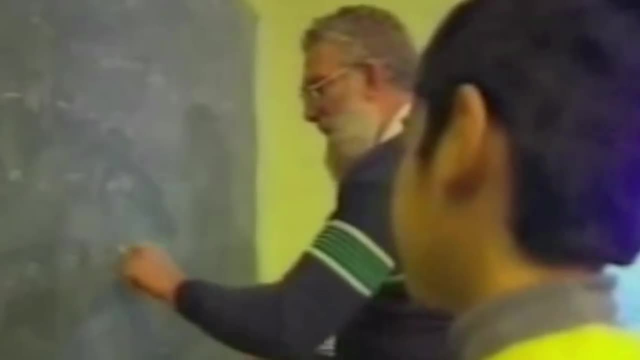 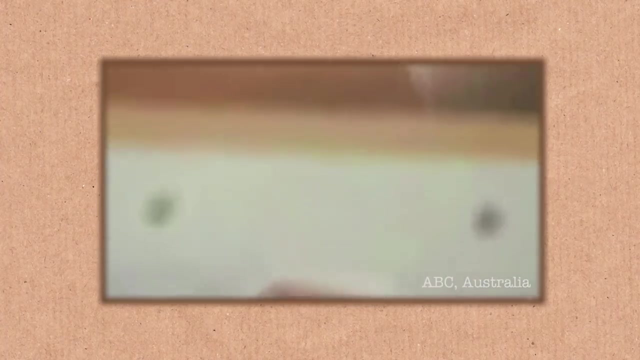 at UCLA at 24.. I enjoyed it. I mean when I was a kid I mostly enjoyed doing maths and geeky things and so forth And, you know, being accelerated and going to uni that early. you know I was. 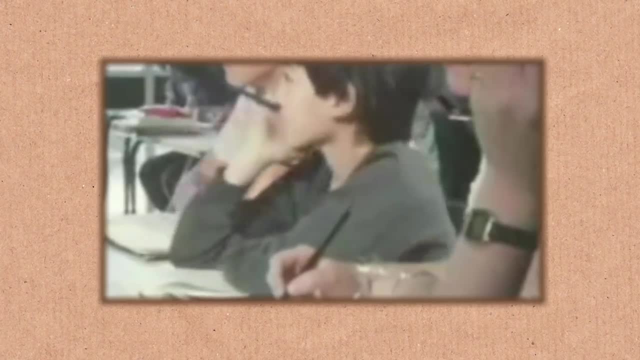 around people who were older than me but had similar backgrounds. So we were absolutely at sort of the same level mathematically. So you know, these people were five years older maybe, but you know we're both struggling with the same homework assignments, We both. 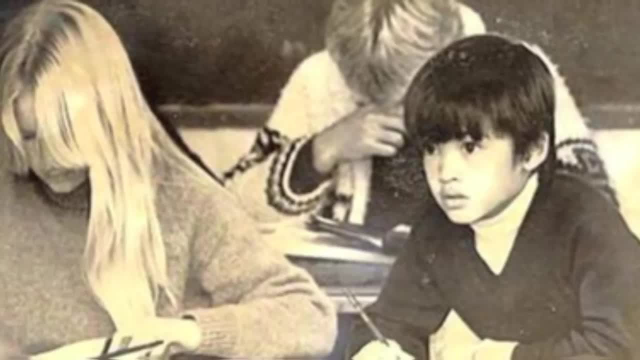 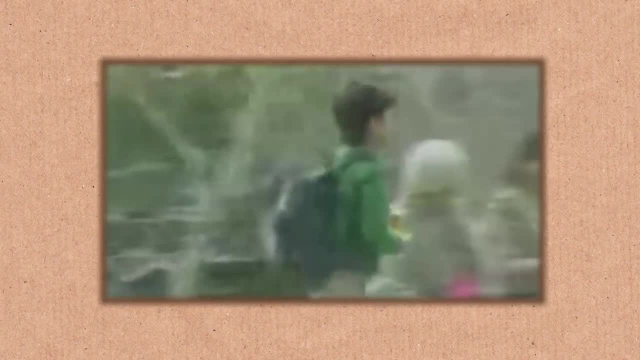 like to talk about various math concepts and so forth. So I felt at home, you know. So I did miss out on maybe sort of the regular high school experience, you know. So I didn't go to too many, you know, high school social events and so forth. I did a lot of that actually. 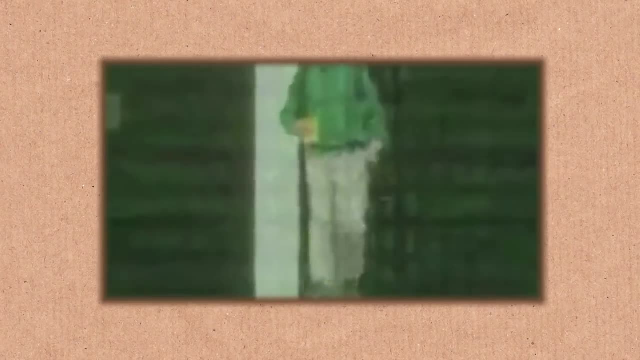 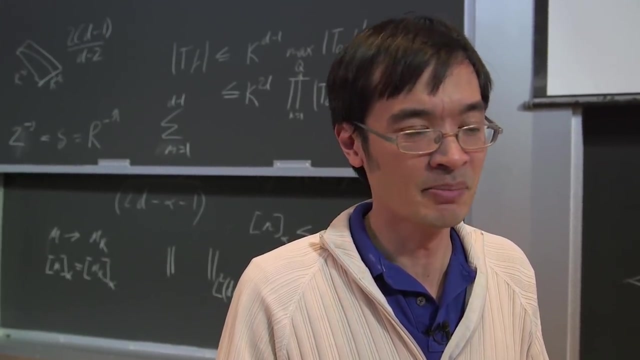 once I was in grad school in Princeton, you know. So then I hung around people my own age and you know. then I partied and so forth. So I sort of had a slightly reorganized childhood. It worked out well for me. 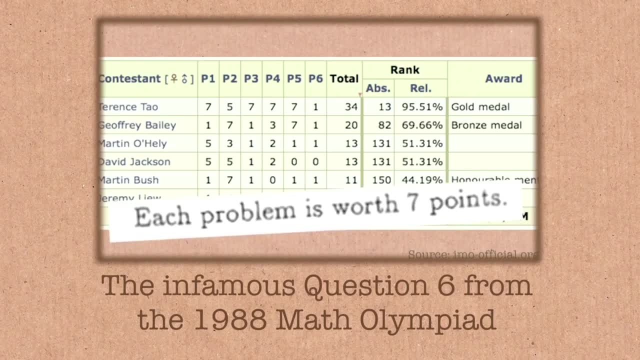 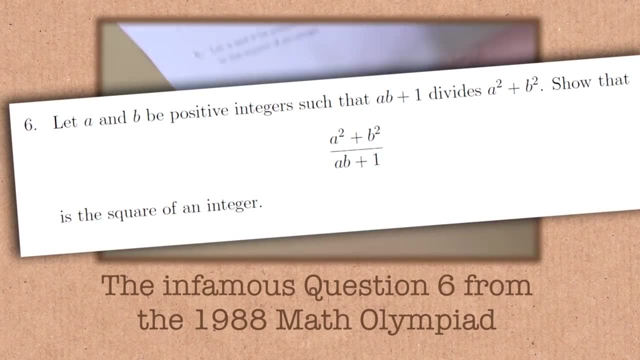 And I have to say Terence Tao was competing there and he only got one out of seven. Let's actually cut Terence Tao some slack. The Fields Medalist, the guy who's like coming close to solving the twin prime conjecture- It's actually pretty awesome because he was only 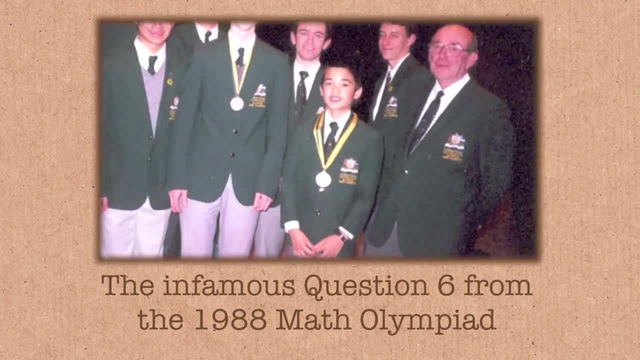 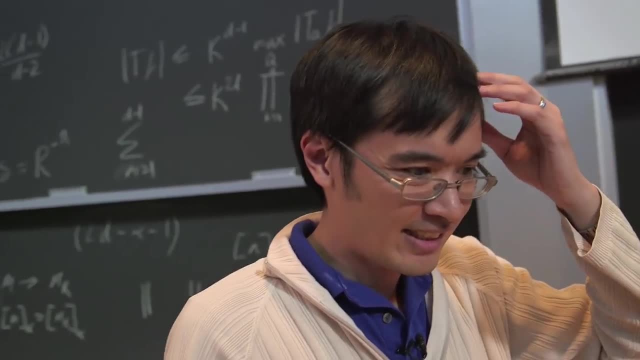 13 years old. He holds the record as the youngest person to ever have won a gold medal. There was this question six, Oh yeah, yeah, yeah, That's a famous question. yes, What's your recollection of it now, and why? And you didn't get it right. 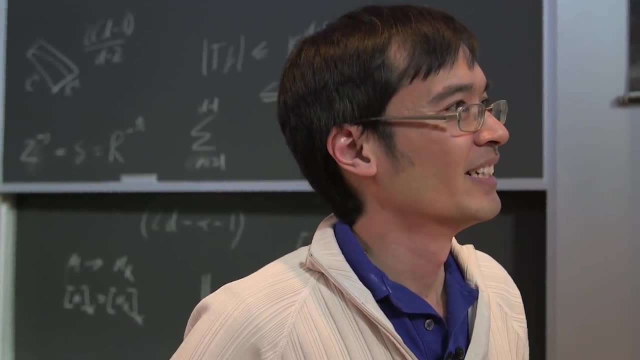 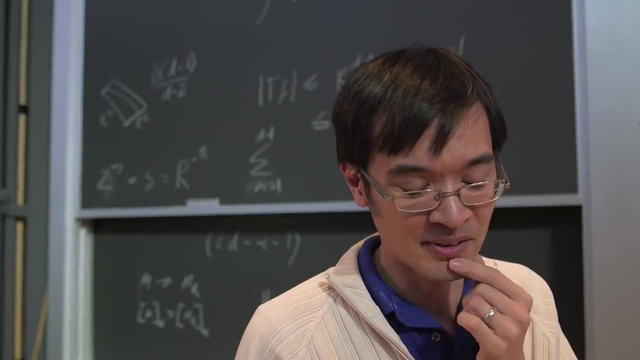 No, I did not get it right. How do you feel about it? Well, you know, you win some, you lose some. Oh boy, It's so long ago now I don't remember much about it. I do remember once, the Olympics was over, I found out that some Romanian woman 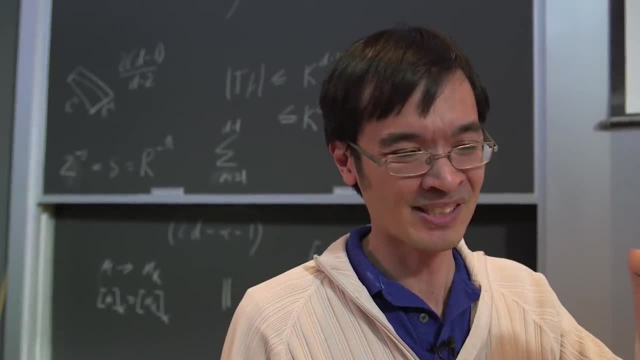 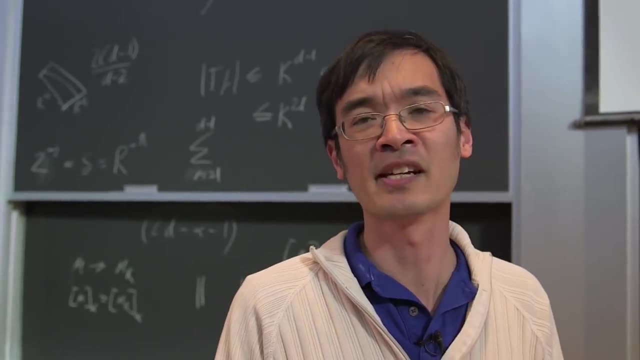 had solved the question and I remember searching out for her because it was really bugging me that I didn't know how to solve the question. There was a special trick to silver which at the time was not a standard trick. that was taught. You have to use the method of. 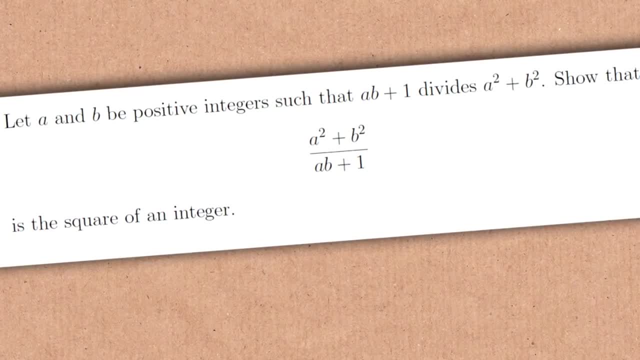 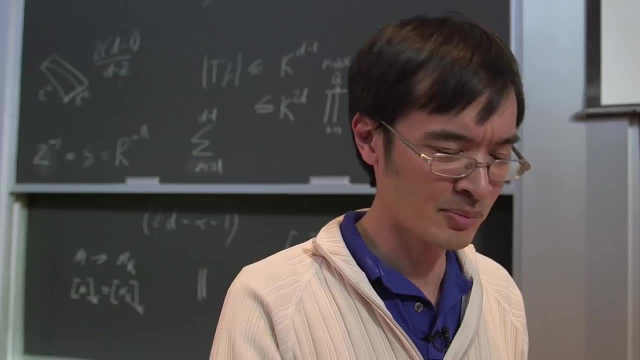 descent? I forget the exact question. yet You have to show that something could not be a perfect square- It was always a perfect square- and show that if it wasn't, you could find a smaller kind of example and a smaller one and a smaller one. I think nowadays it's become part of. 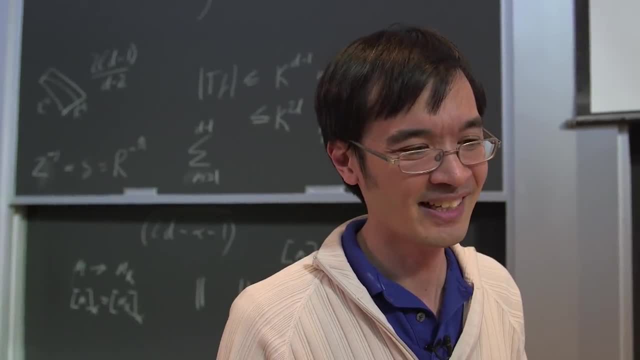 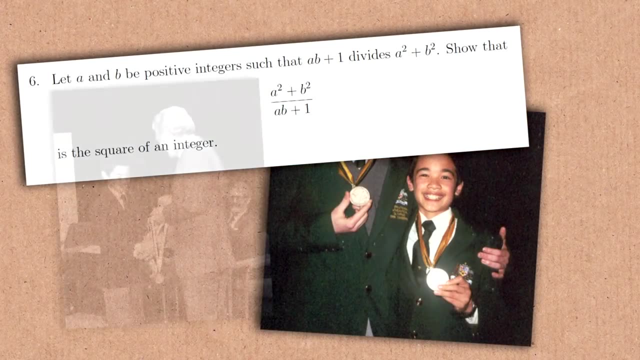 the standard training. They all know the trick now. but yeah, Were you competitive? Were you the sort of boy that would get upset about it? or was it just a fascination? I just want to know the answer. or were you angry that you didn't get? 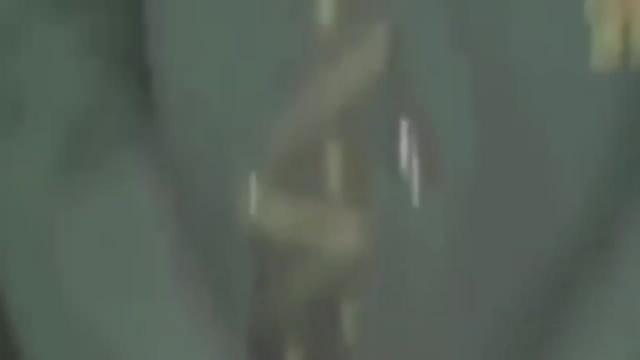 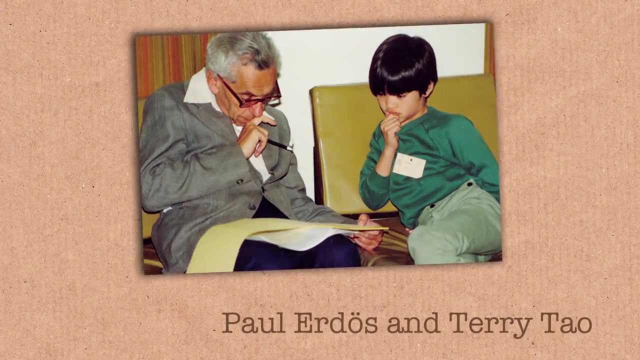 it. I think I was more obsessive than competitive. Yeah, I mean, certainly I was a bit angry at myself for not getting it, but I wanted more to know the answer than to win. I think There's this famous image of you with Erdos, this photo, which is a great photograph, People. 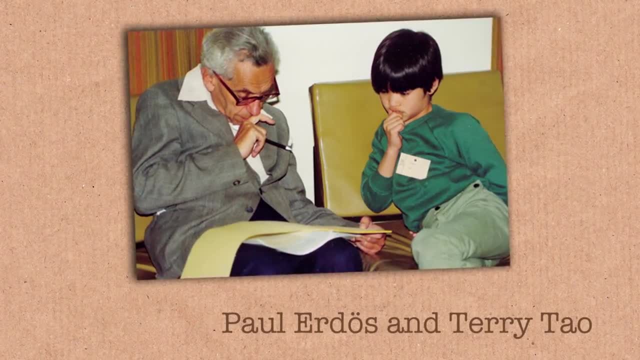 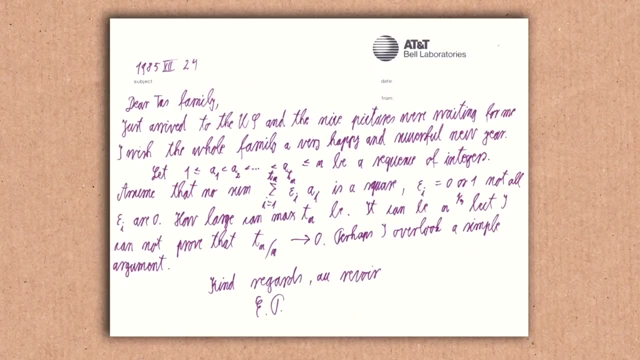 want to know what you're discussing in that picture. What's going on there? I think he was giving me a maths problem, which I think I even know what it is, because he did send me a postcard afterwards with what may be the same problem. I have it somewhere. 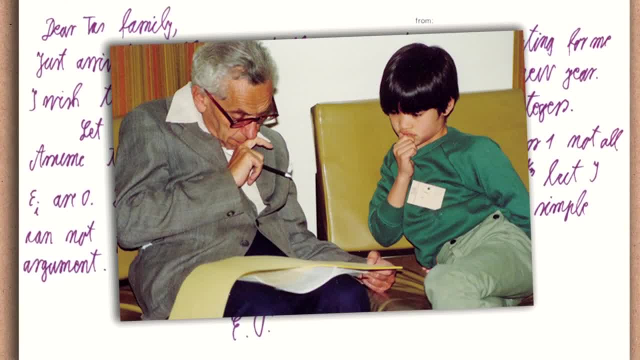 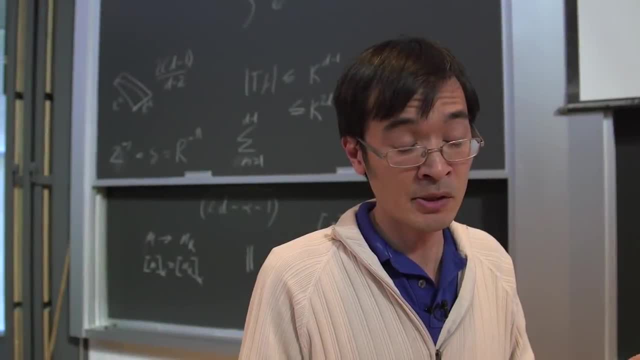 Yeah, I think it was some maths conference in Adelaide. Yeah, I was like 10 or something. I don't remember why I was there. Maybe some maths professor at the University of Adelaide told me to come. I understand he was always very good at speaking to mathematically gifted. 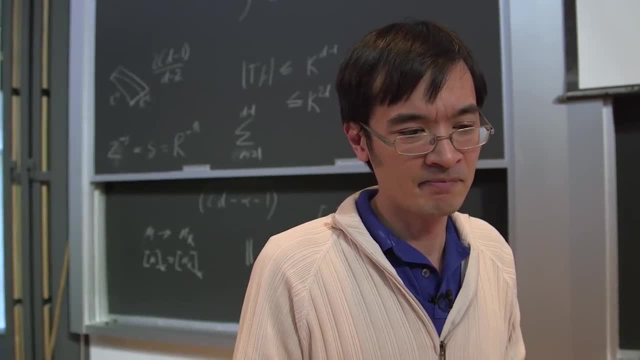 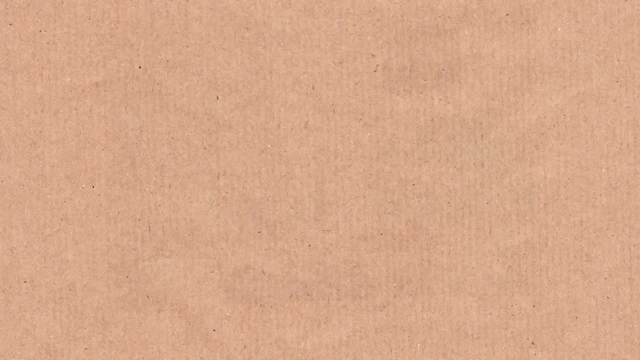 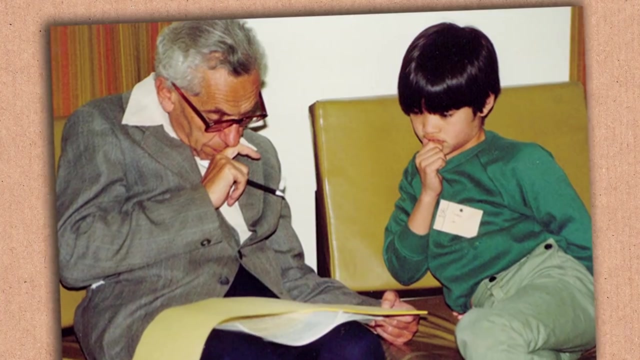 kids. I don't remember much about our conversation, except I remember I really felt like I was being treated like an equal. He wasn't condescending or anything, It was just a very pleasant conversation. Now that the audition has passed, it does have some sort of value for me. 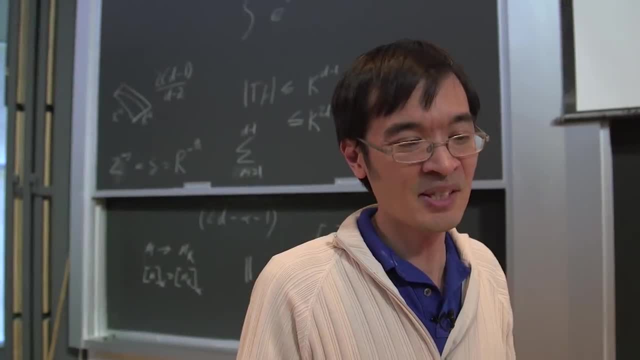 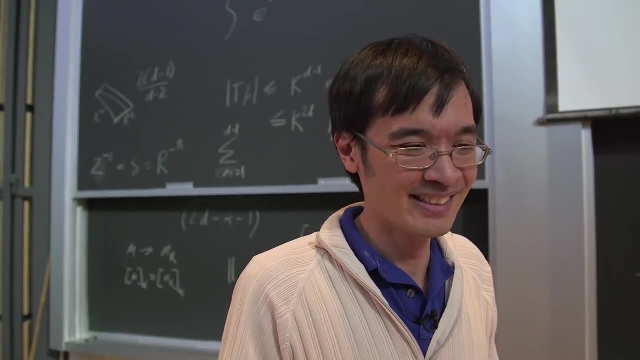 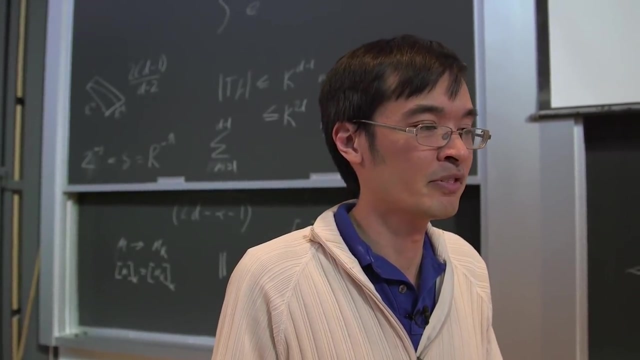 I certainly wish I'd paid more attention to him. actually I'd heard of him as a child. To me he was just someone who liked talking math to me. That was great. He did write me a letter of recommendation for Princeton later on. He did help my career directly. 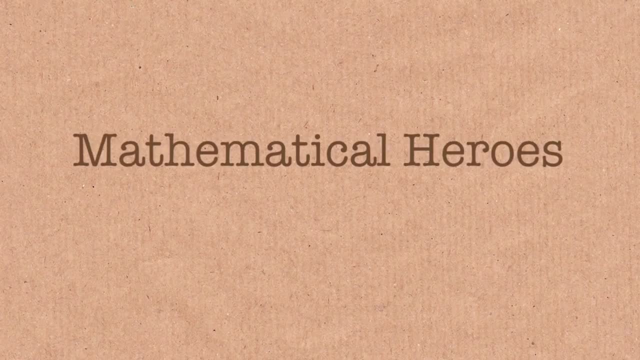 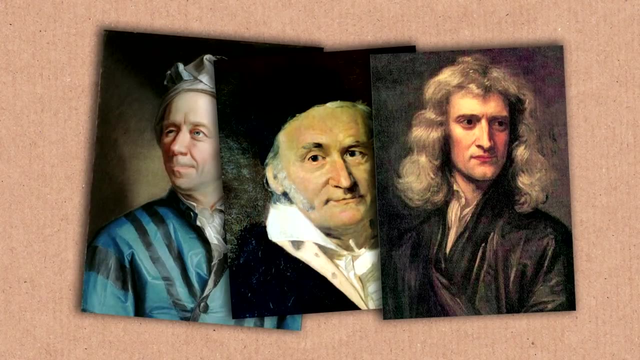 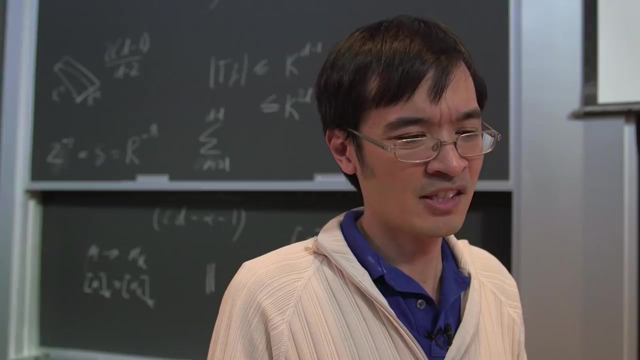 Did you ever have people you looked up to and thought they were the top guns? Not really. I would learn about Euler and Gauss and Newton and so forth, but I didn't really have a good sense of what was the most important. I didn't learn the why of 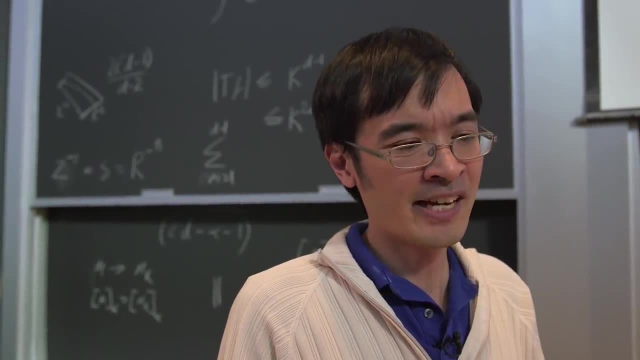 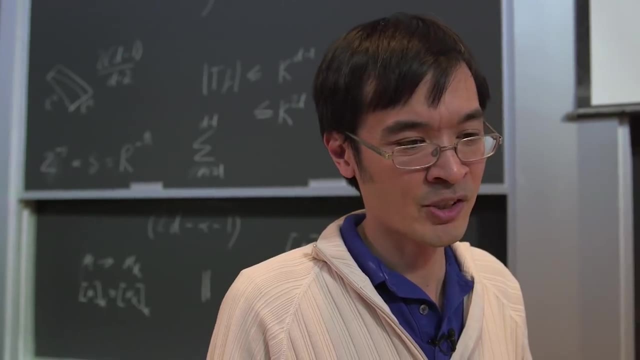 mathematics until a while later. I remember when I was learning calculus I thought that the most important mathematician in the world must be Taylor. Taylor's name appeared everywhere in undergraduate calculus, Taylor expansion, Taylor's rule and so forth. He was a good. 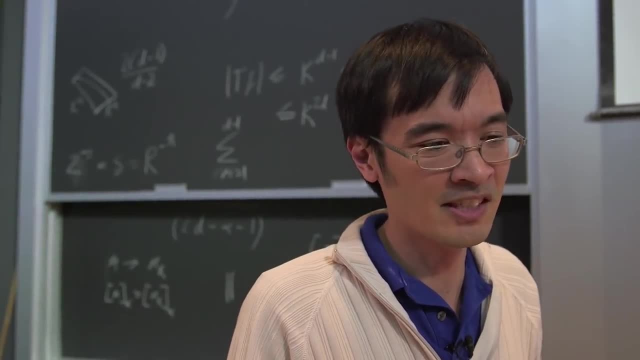 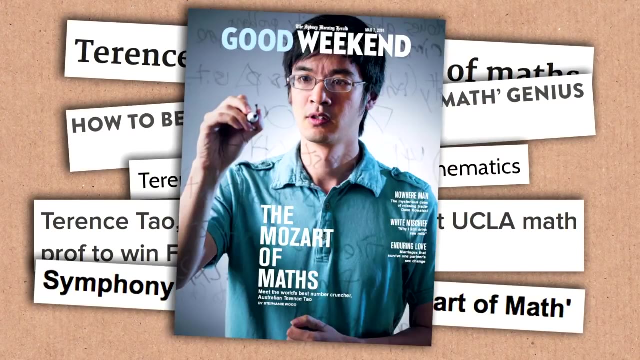 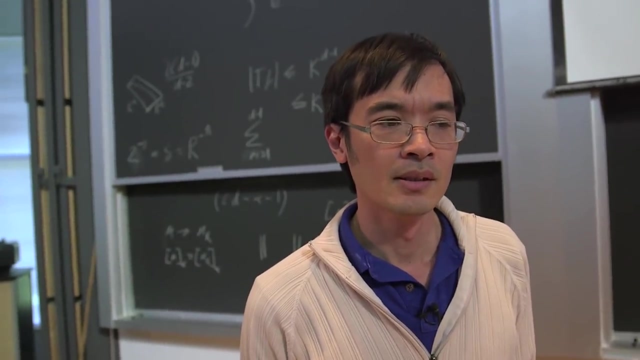 mathematician. There are many other people who did good stuff. it's just not taught as much at the undergraduate level. When you're doing mathematics, do you use any kind of visualisation in your head? What does it look like in your head when you're doing math? 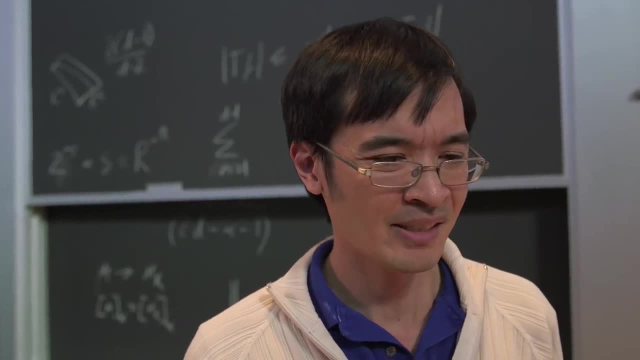 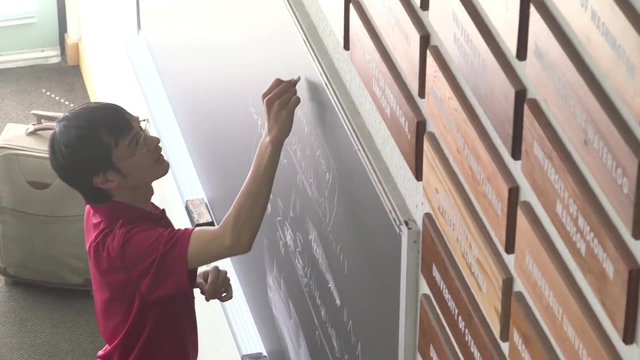 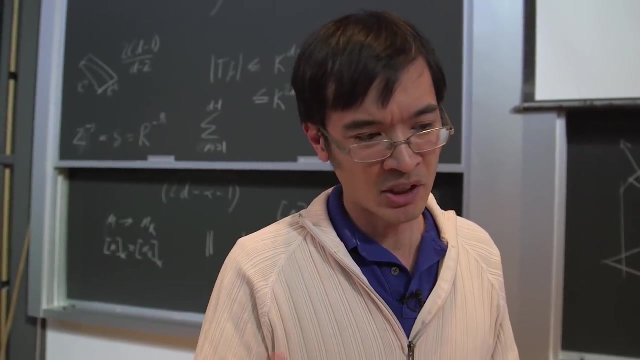 It's a bit hard to explain. It's always a combination of thinking inside your head and speaking out loud and working on the board. You do try to isolate the simplest metaphor or something for your problem. How can I explain it? For instance, I do a lot of estimates. 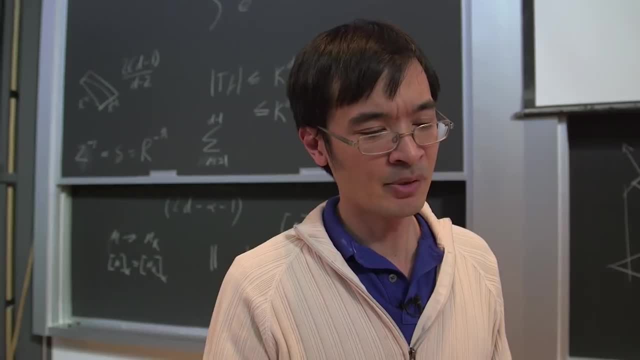 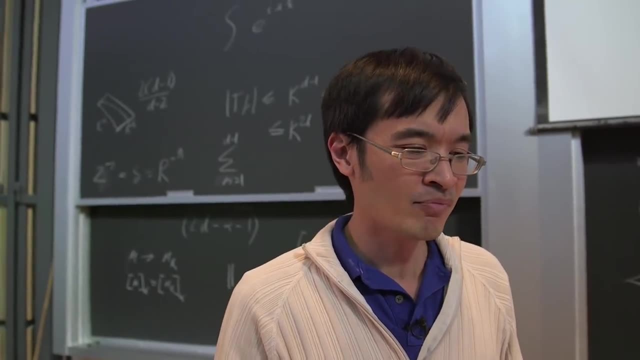 I always want to prove that x is less than y. Sometimes it helps to think of this as an economics problem. You have a budget of y and can you afford x. That way you start thinking economically. The way you prove an equation. 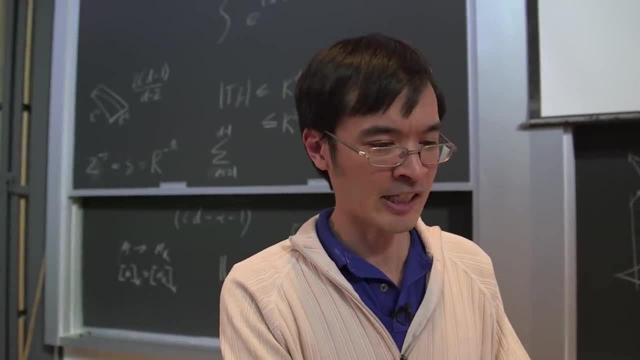 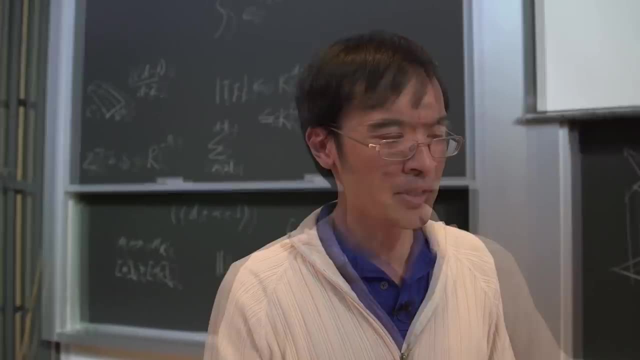 there are inequalities like x is less than y. Normally you try to first find x by z, then z by w, then w by y, and so forth. This is like trading in one item for another item. You get a sense of what inequalities are good deals for you. 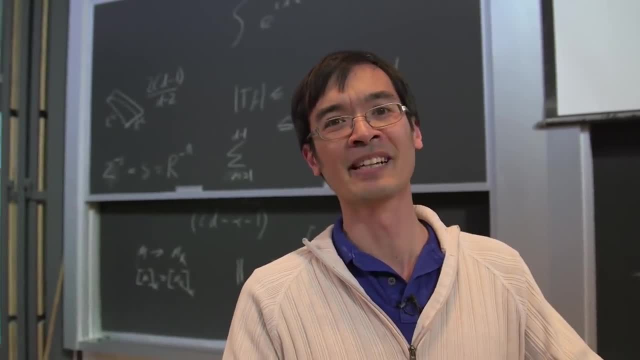 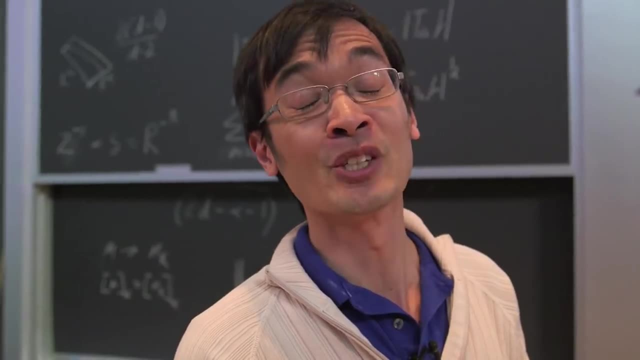 You're getting your bang for your buck, Which ones are really wasting your money. Sometimes, utilising your financial intuition can be helpful. Algebra and topology: Those have always been my weakest areas. I've only been able to get a handle on them. 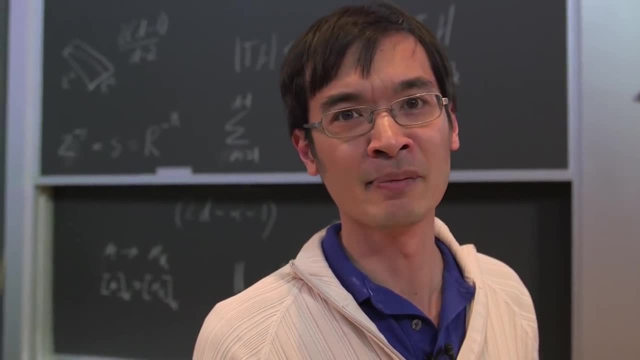 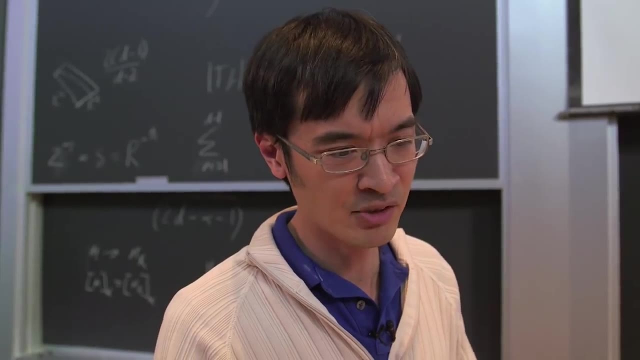 Generally by translating them into other types of mathematics- Geometry or analysis I have a better handle on. I certainly don't claim any mastery of all of mathematics. I think nobody can do that, not since Hilbert. The work I'm proudest of is almost all joint work. 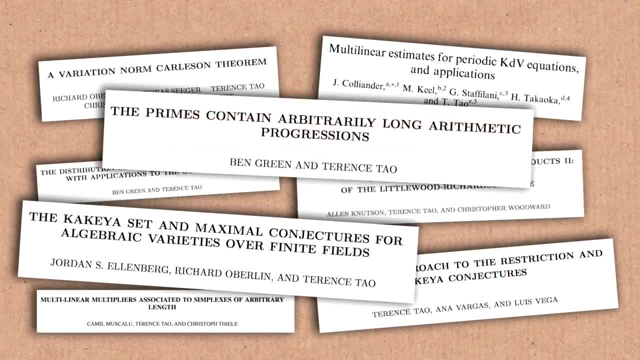 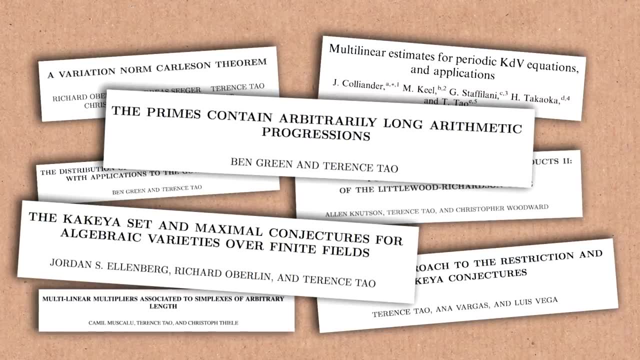 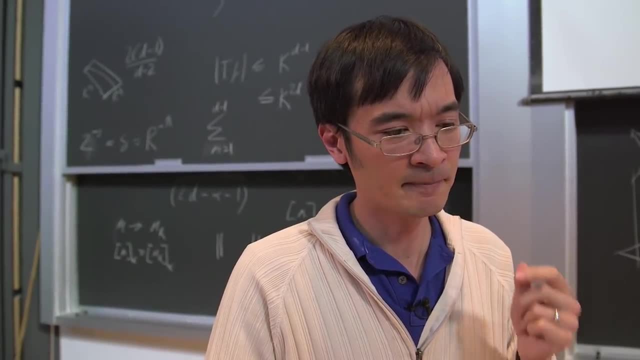 Nowadays most of my work is joint. It is really fun to talk over a math problem at a really high level with a co-author who is really on your wavelength, understands what you're thinking, Saying things out loud. it forces you to think at a more organised level. 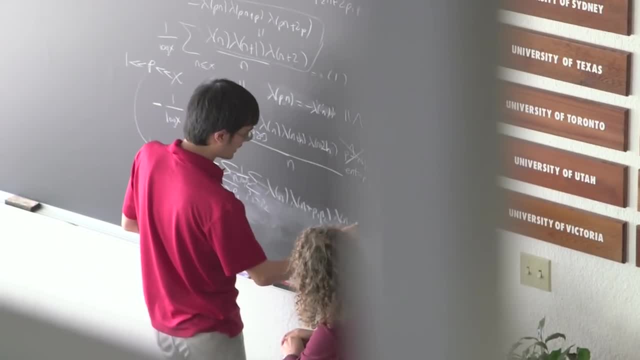 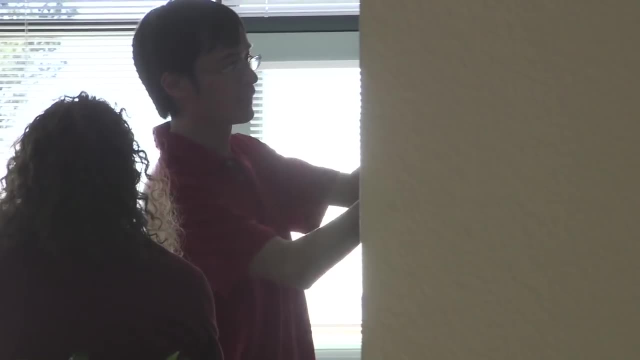 than in your head, where it can be a bit jumbled and vague. It's just more fun. You can go back and forth. If you're stuck, maybe your co-author has a suggestion. If he or she is stuck, you can make a suggestion. 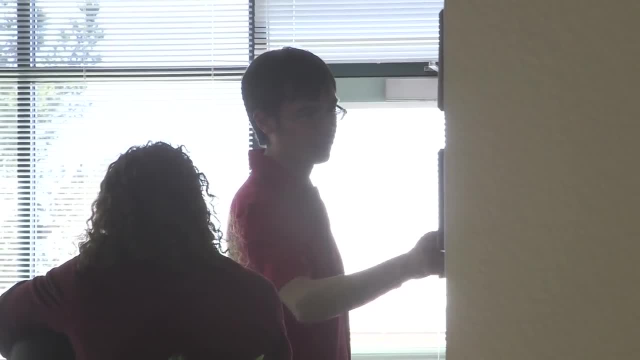 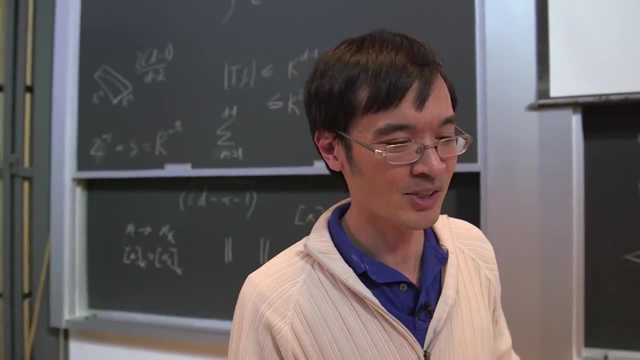 You at least guarantee one other person is interested in what you're doing. When you write a paper by yourself, there's always a nagging fear at the back of your mind that maybe no one will care about this. You at least have one person to talk about it with. 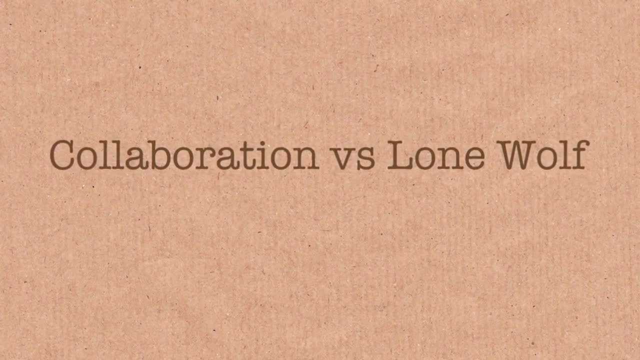 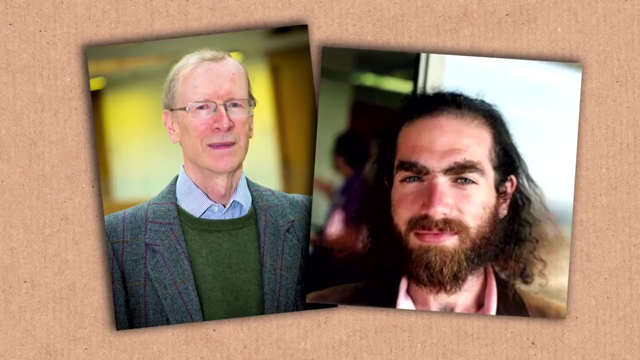 What do you think or feel, or what's your impression of those mathematicians that go the opposite way? Andrew Wiles is an obvious example: the mathematician who works in solitude. How does that impress you? What he did was very impressive. You need both. 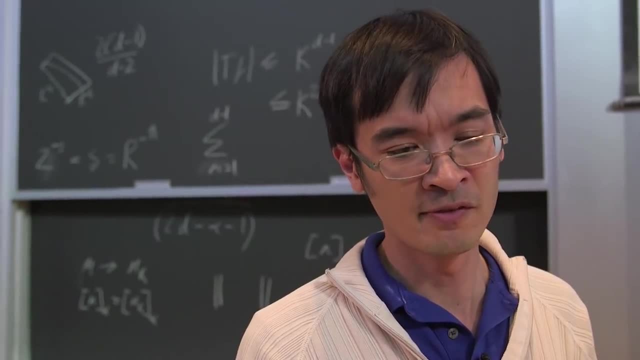 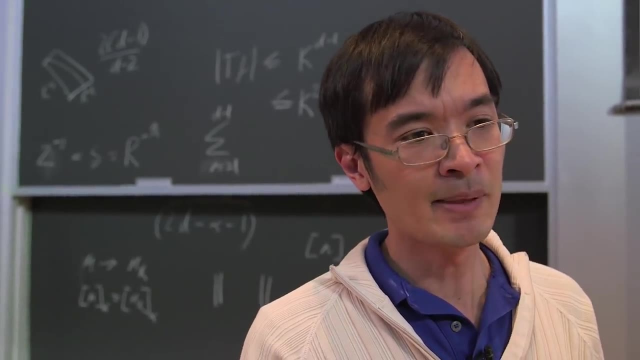 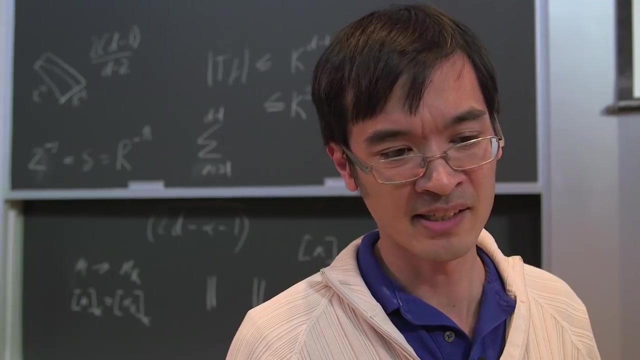 You need people who focus very, very hard on one very narrow problem and, working for years, become a very deep expert. But then you need the people who can connect things from different fields. I make my living by understanding one thing. I can't do that without applying it to field X.